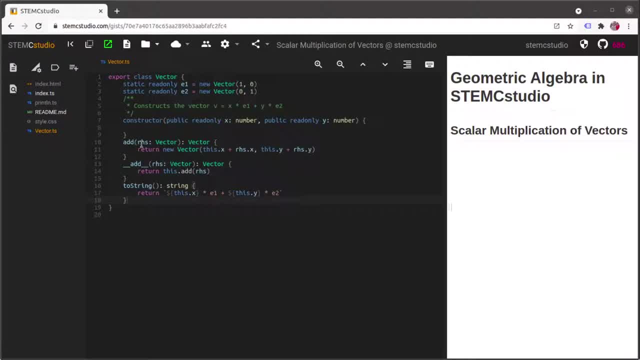 use a simple pair of numbers. We added a method for adding two vectors together and we provided the corresponding method that did operator overloading, And then, finally, we added a two-string method that would provide a string representation of the number. What we'd like to. 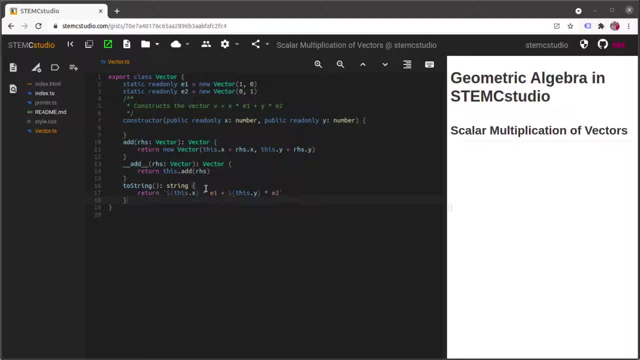 do first is we would like to improve the documentation a little bit. So if you start over different parts of the class, like hovering over the vector here, you'll see it's not producing any documentation. The constructor is, and that's because of the JavaScript or the Java. 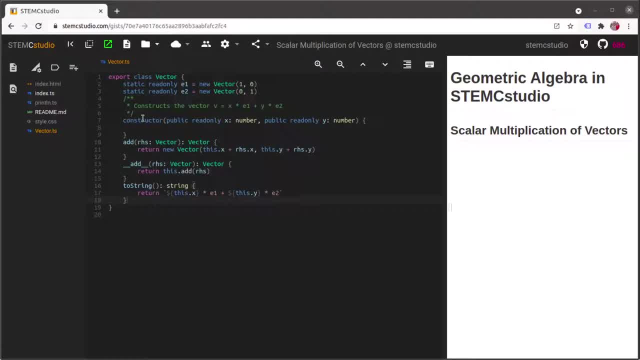 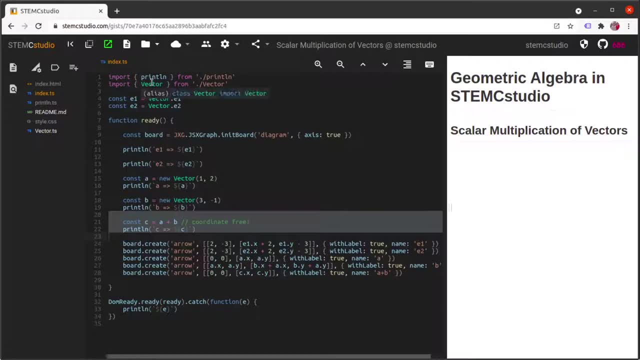 doc style comment that we have here but it's actually not complete. And then further if we go to where we're using it. if you hover over various things like the vector itself- the basis vectors of the vector are not nice- We don't get any extra information. The constructor's not too bad, Okay. 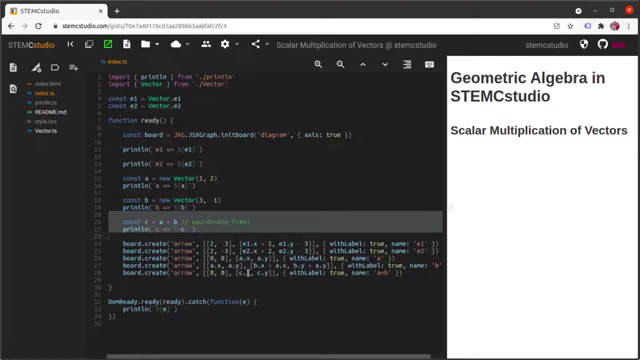 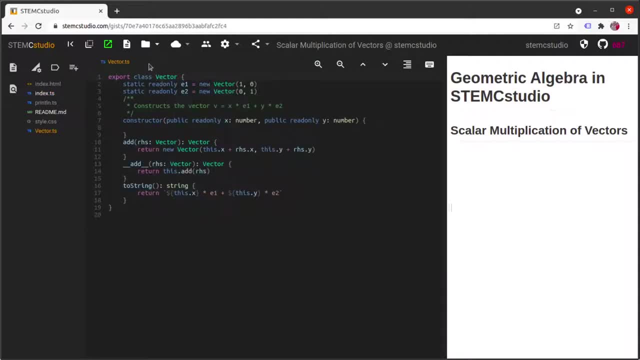 And, yep, even the properties are not giving us a lot of information, So let's go and fix that. We'll right-click on vector, go to definition, And one of the things that we can do here is just add a JS. 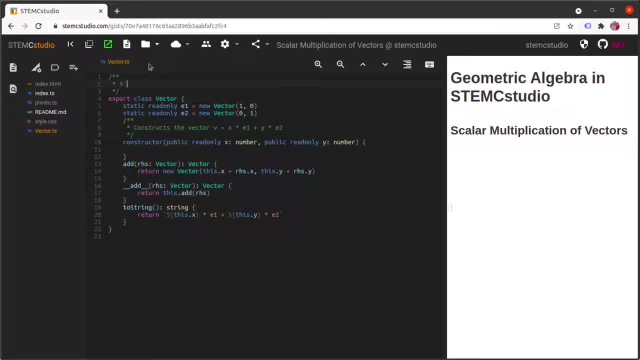 style document at the top of the class and we can say a vector in two dimensions. I won't say much more than that at this point because we have some dimensions. i won't say much more than that at this point because we actually haven't really. 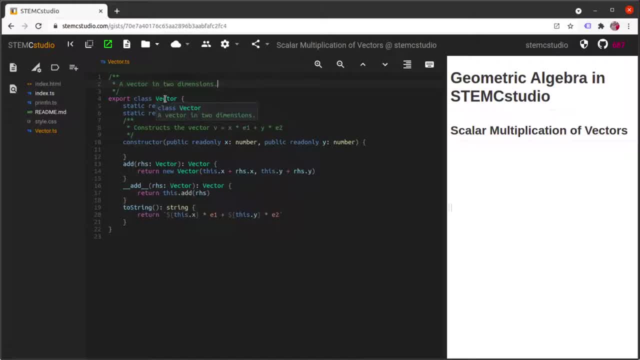 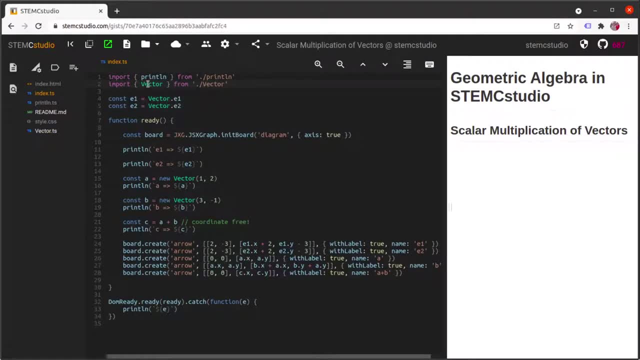 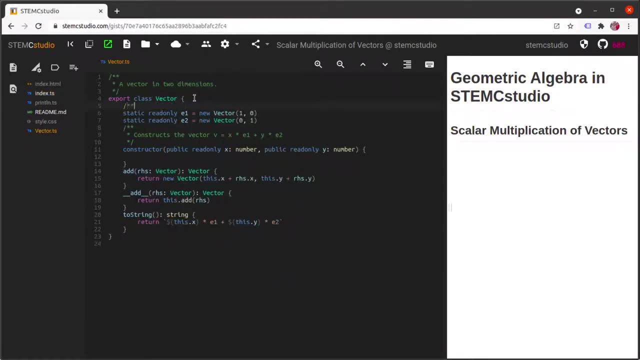 defined much more for this. if we hover over vector we see it says a vector in two dimensions. that's great. if we come back to indexts and hover over that, you can see we've got a little improvement there. okay, let's take a look at these e1 and e2. we'll give that a little js doc document, okay, so 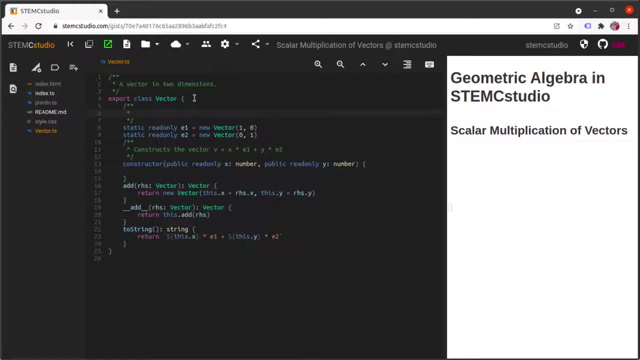 what is e1? e1 is um, a basis vector, a basis vector, and uh, it's kind of really hard to say what. what else we should say about this here in the, let's say, x direction. similarly, we'll say here: in fact, i'm going to change this- 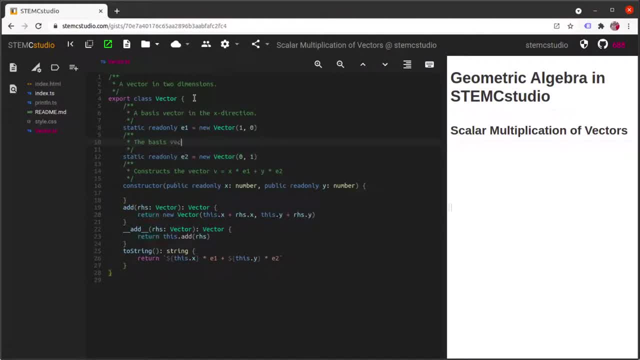 thing and make it the basis vector in- uh, even better, even the basis vector corresponding to the y coordinate or y coefficient. i think people say coordinate, coefficient component. none of them is really very satisfactory, um, but actually i think that in some ways coefficient actually says what we want much better. 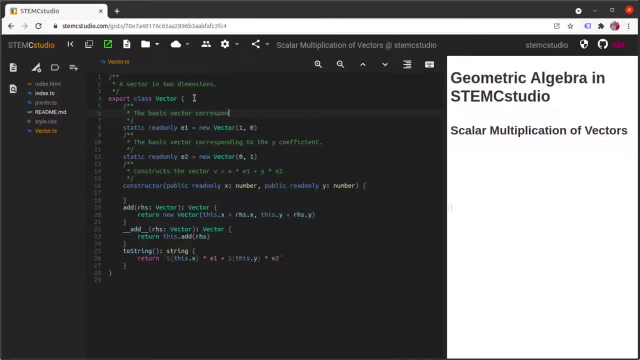 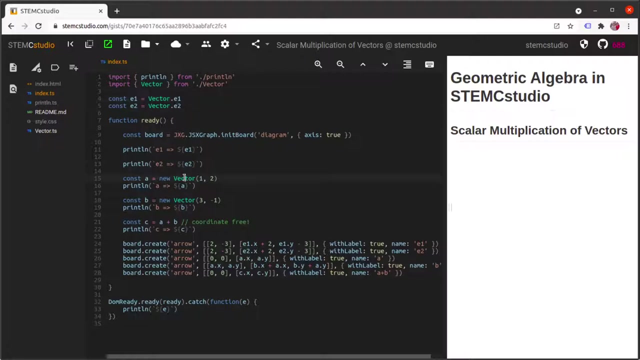 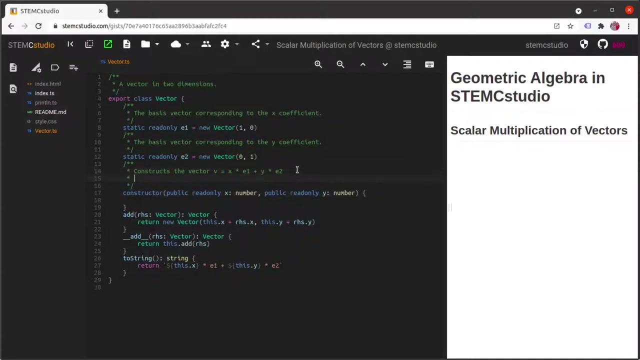 so the basis vector corresponding to the x coefficient? okay, so we can hover over these now and that's a lot better. hover over these, those are a lot better. okay, what about the constructor vector? so the constructor takes parameters x and y, but we haven't really described what those are. so 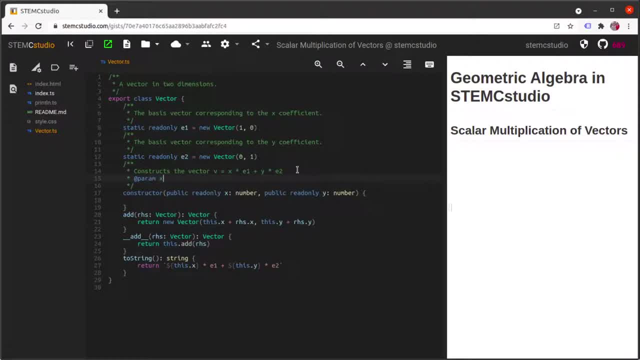 the syntax for that isanksine param, the name of the parameter, and then we can say here the- we'll use lowercase- the coefficient corresponding to the e1 basis vector. okay, the coefficient corresponding to the e1 basis vector. okay, the coefficient corresponding to the e1 받고. there's two parameters. 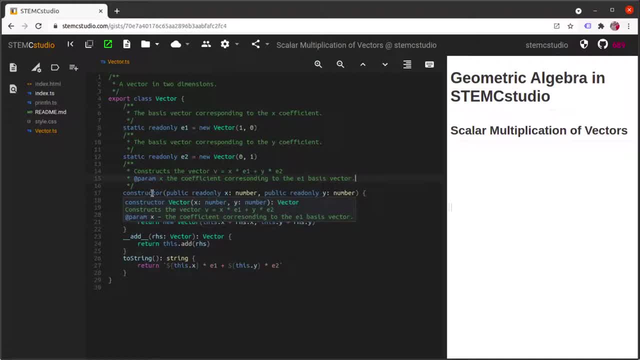 corresponding to the E1 basis vector. If we hover over this, let's unparam the coefficient corresponding to the E1 basis vector. Let's do the same for y Coefficient corresponding to the E2 basis vector. Okay, so, constructor, a little bit. 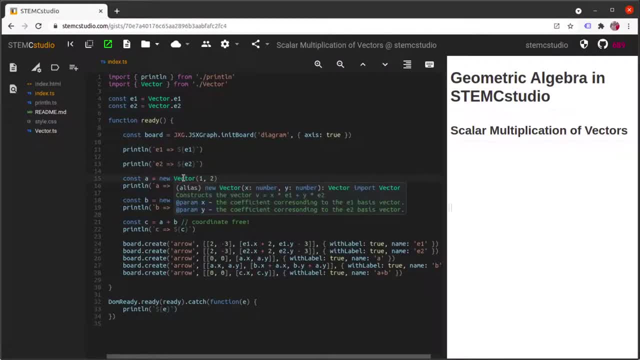 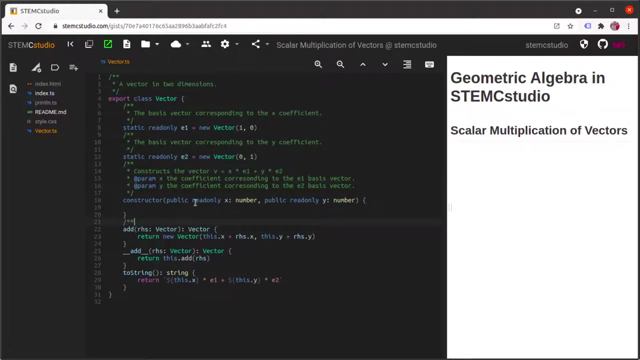 more self-explanatory here. We will actually, in the future, we're going to try and discourage people from using this constructor and instead have them use convenience methods. but that's down the road, Okay, so what else should we document here? Well, we probably should. 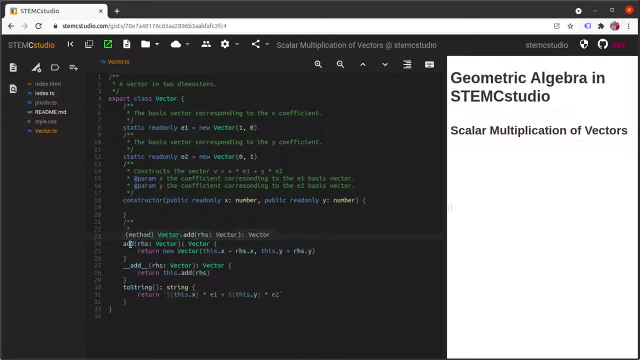 document, the add method, because you can actually use the add method directly. This method here we don't really use directly, It happens through operator overloading. So you that really shouldn't be seen. So here what we can say is, let's say, we can say: 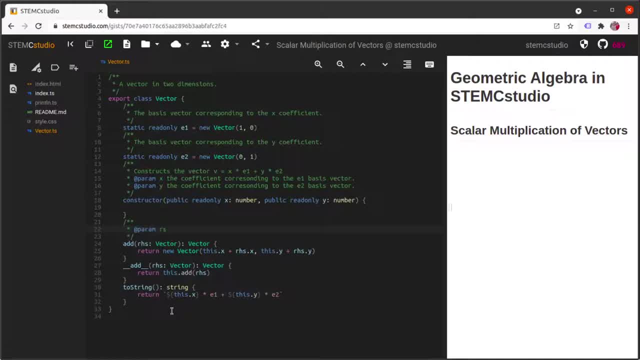 well, there's obviously a parameter and right-hand side and that's the vector. to add to this vector And we could perhaps use the returns, keyword returns, This plus right-hand side. Okay, And there's no need to say that this is a vector, because 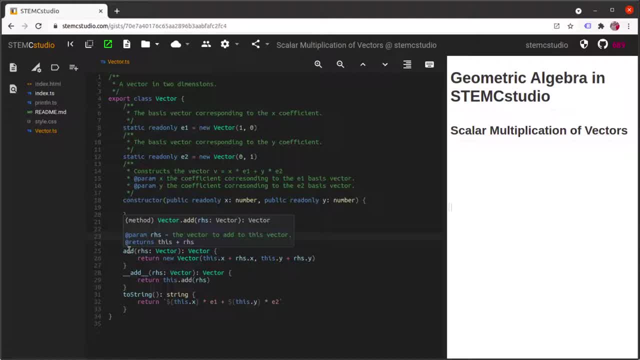 it's actually built in to the type definition. Okay, So it just returns this right, And you might say a new instance. What I'm trying to suggest here is that it doesn't modify the type definition. It doesn't modify this vector. What else can we do? Two string? Yeah, we can use two. 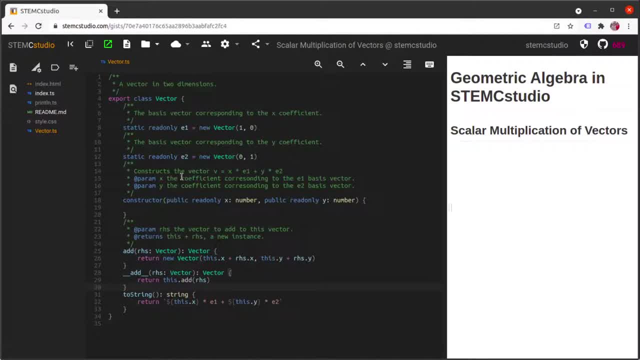 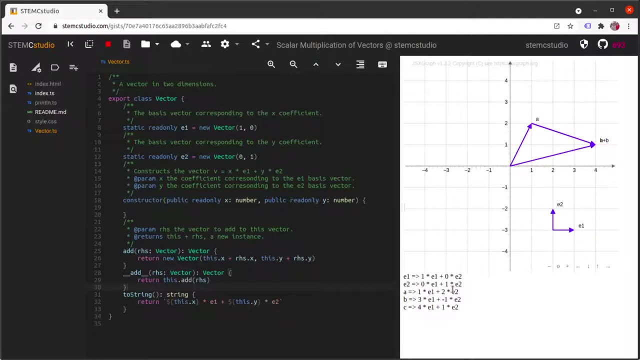 string. I'm not going to worry about that right now, but you get the idea, Okay. The next thing we want to do- let's run this- is: we want to improve the printout here So it looks a little bit more natural. Okay, So let's run this And we want to improve the printout here So it looks a 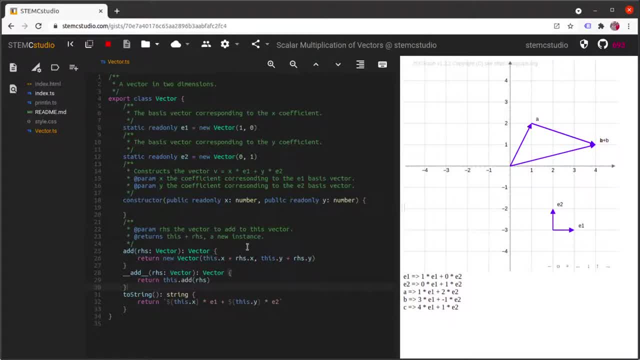 little bit more natural. Okay, So let's run this, And we want to improve the printout here. So what we're going to do is we're going to use MathJax for that. So MathJax is a library that can take. 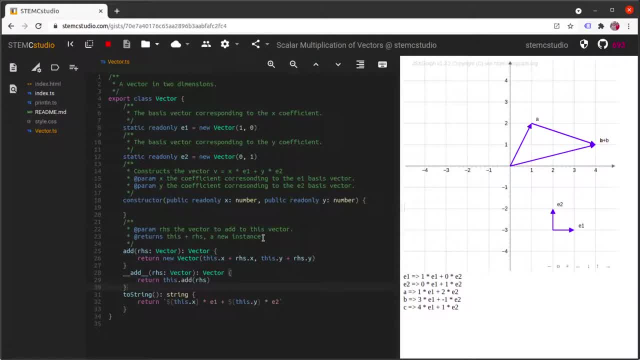 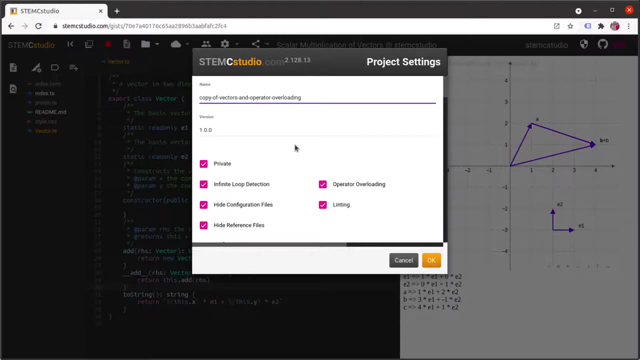 mathematical expressions in various formats And it can render those in a sort of more natural mathematical syntax. So to do that we first need to make MathJax available to our project. So we head over to project settings. You can see, here the title is not really very appropriate. 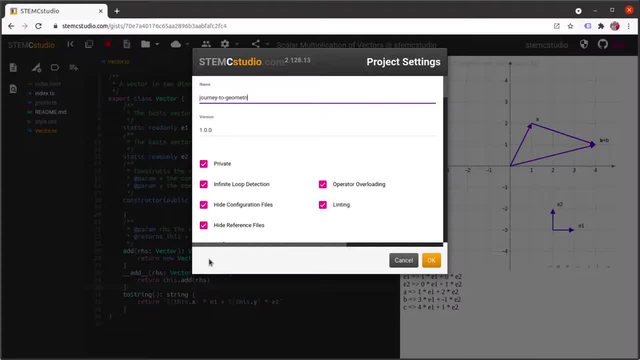 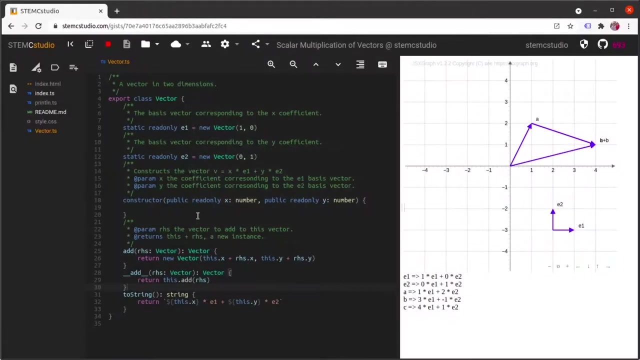 Journey. I guess that'll suffice for the future. It's not really important. This is just maybe something that will become more useful in the future. Let's find MathJax here. There's MathJax, And we'll take the latest version, which is 3.14.. Okay, All right. So to actually use MathJax, there's two things. 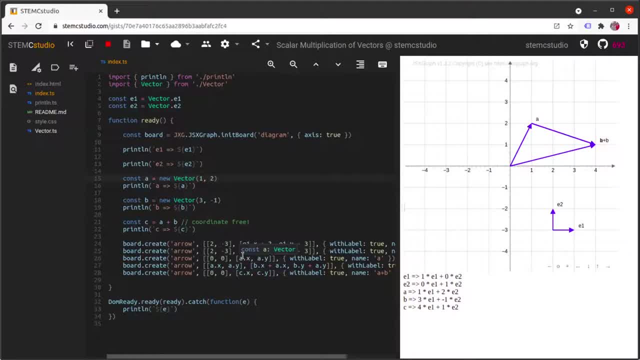 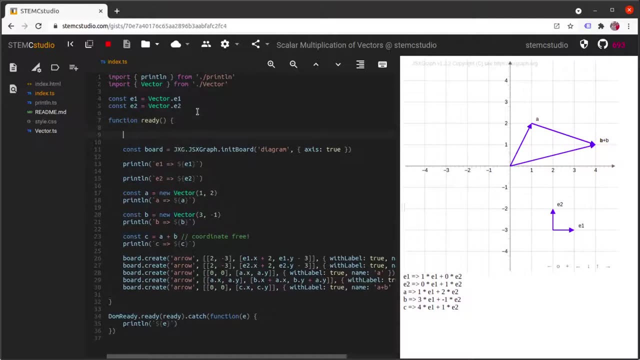 that we'll have to do. One is that we want to use it for our own print line statement down here, And the second is that we want to use it in JSX graph. Now, to use it in JSX graph, we basically have to prepare JSX graph. 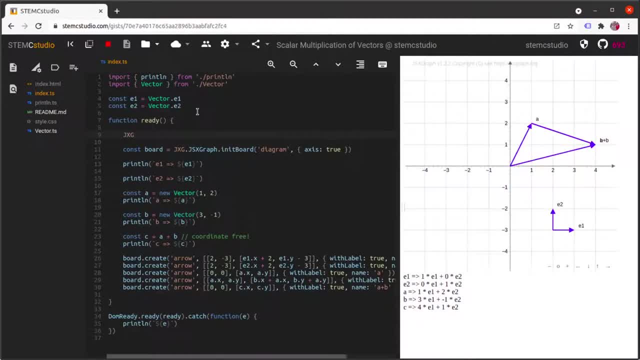 a little bit. So the way to do that is you type jxgoptions, And then it's text, And then dot And use MathJax And we say true, Okay, So that's going to set us up correctly. now You'll notice we've got this. 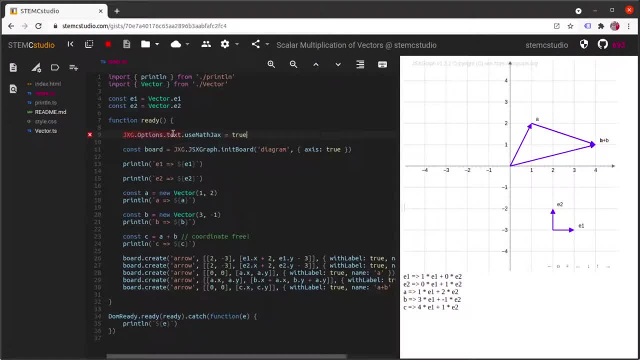 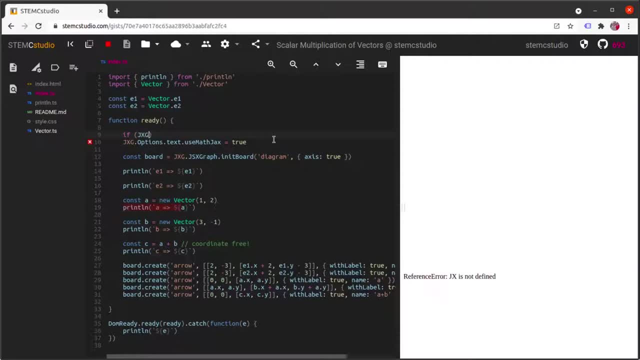 sort of type behavior saying, hey, text is kind of optional, It may not be defined. I'm not sure here whether this is sort of really to be considered an error in the way that the system is typed. I'm not quite sure what the correct semantics of this API should be, And so 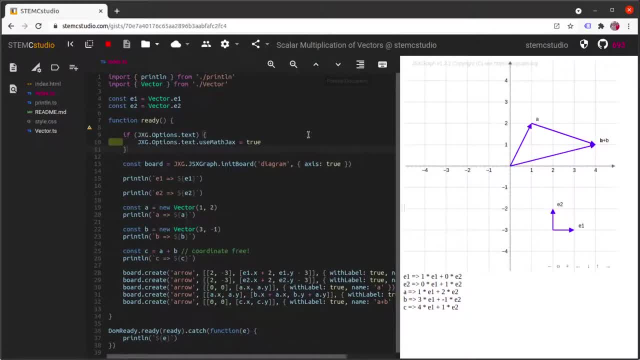 this may not be the sort of the correct ultimate fix, But what we can do here is we can just make this conditional And TypeScript knows that if this evaluates to true, if it's truthy, then text is safe to use. It's just text options now And we say: use MathJax, true, Okay, The final thing. 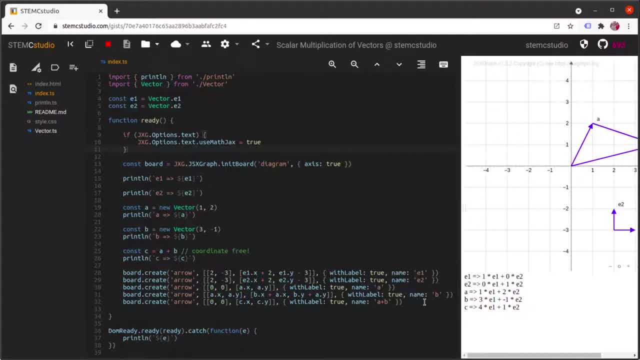 that we then need to do is we need to sort of surround our, our usages of our names with a sort of an escape sequence which indicates that it is MathJax. So the way to do that is a double backslash, square braces, double backslash and then close. 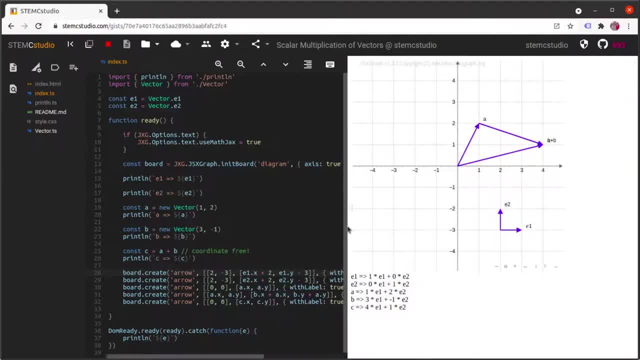 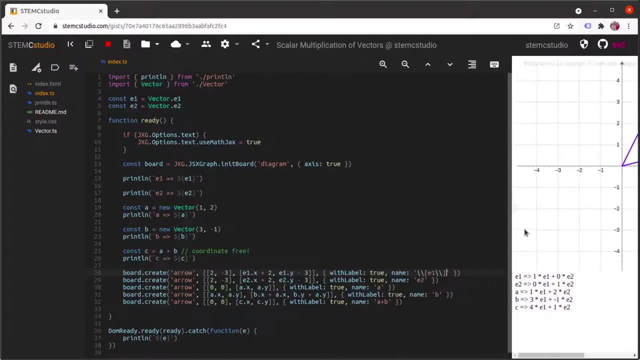 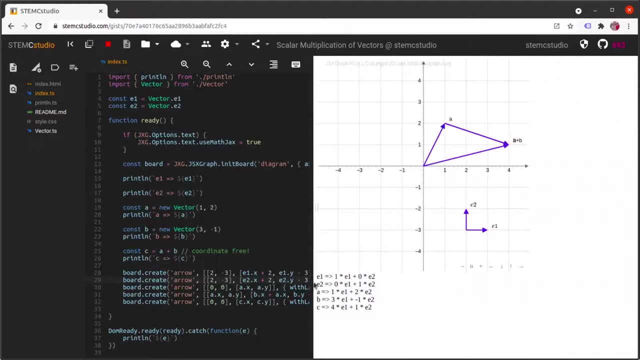 square braces. Okay, And we may need to stop and start, but actually, no, it looks like it's recomputed here. So we've got E1 coming out now the way we want it. You can also use $$, I think. And yeah, there it is, We've got E2.. Now, actually, we can do. 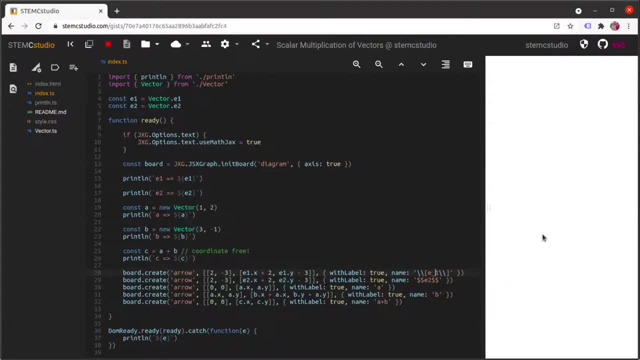 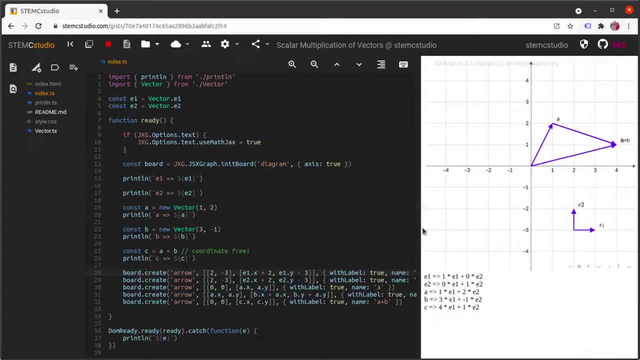 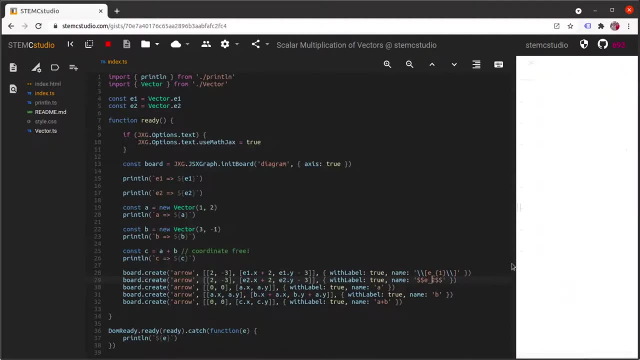 obviously a lot better than this. We want to make it look like a little underscore with a subscript, So to do that, I want to use the underscore and then 1. And you can see it's dropped it down there. That's exactly what we want, Okay, So here would be E underscore 2.. 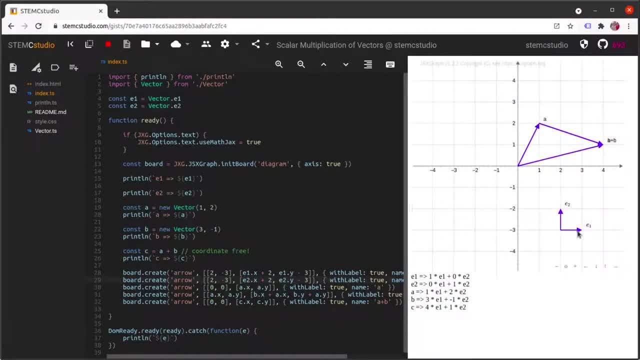 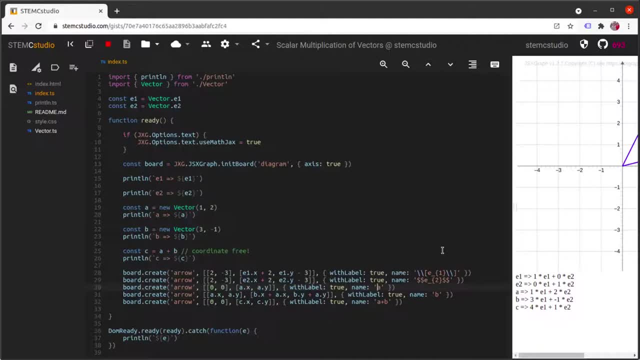 Like that, And just see E1, E2 looks kind of quite pretty, And then let's do the same for A here. So I think for consistency we should sort of stick with one or the other. I'm going to go with actually the square bracket form like that And I'll make this the square bracket form 2.. 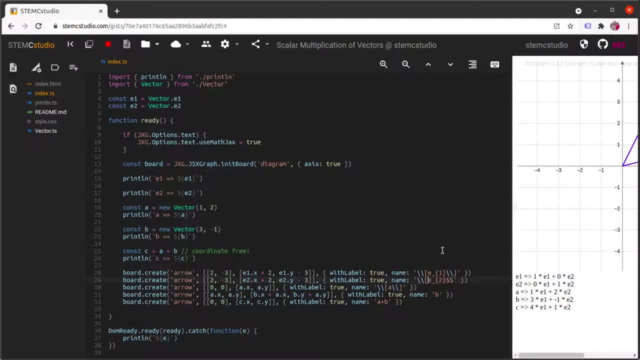 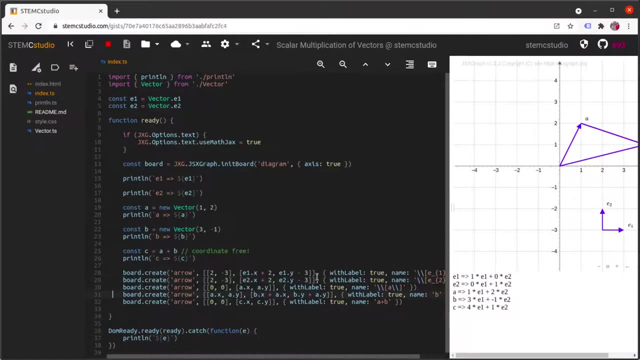 Oops, Do that again. Double backslash, square brackets. Okay, And so are we good there. E1, E2 looks good. A- I'm not going to bother with these other ones, B and C, because we actually won't be using those going forward in our. 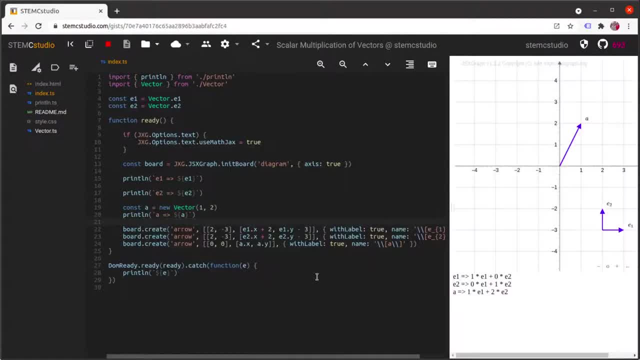 work today. Get rid of them all, Okay. So what can we do, then, to improve this down here? Well, what we need to do is we need to also escape. So we'll do this and close off. Okay, Now you can. 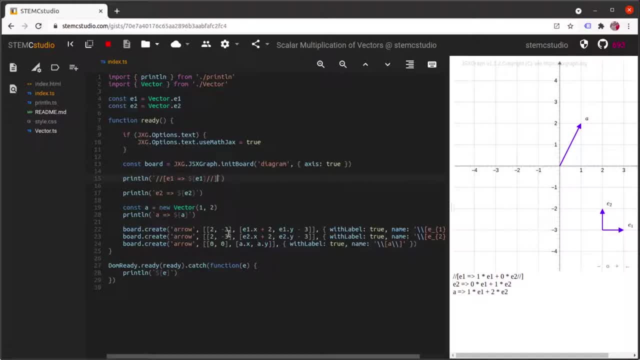 see nothing's really happening at this point. That's because what we need to do is we need to give MathJax a little hint that it needs to typeset Okay, And the reason for that is that recall this DOM ready. MathJax did its initial processing. 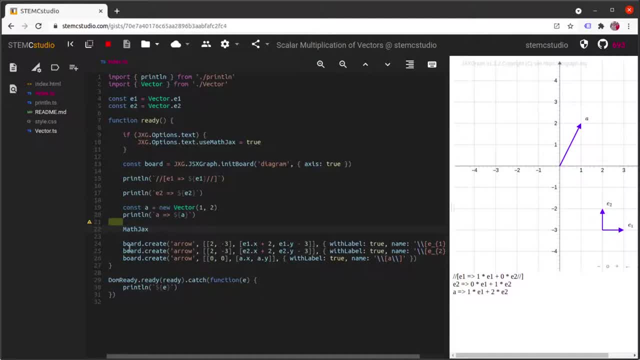 When it thought the DOM was loaded. But now we need to make sure that it's kind of processing at the right time. So you can use typeset. Typeset promise is a variant And you can look at the JSX graph documentation to understand exactly what we need there. Okay, So 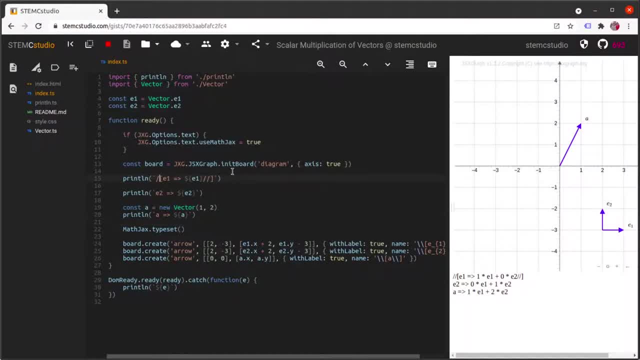 didn't kind of quite work out. I've got forward slashes, Need to have backslashes, And okay, we are getting there E underscore one, So that's looking better. But now what we have to do is we need to go to our vector and modify it so that it's returning a sort of a MathJax-y form. 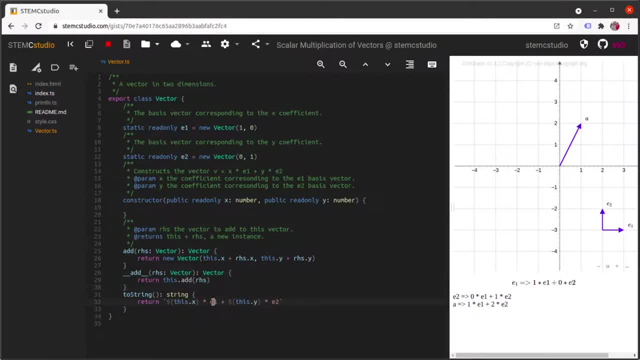 Now, obviously, you could have different kinds of variations here. You could, you know, vanilla, two string or whatever, or two latex or something like that, But we'll do this Looking pretty good. Now, one of the things with MathJax is that you know, we don't really need. 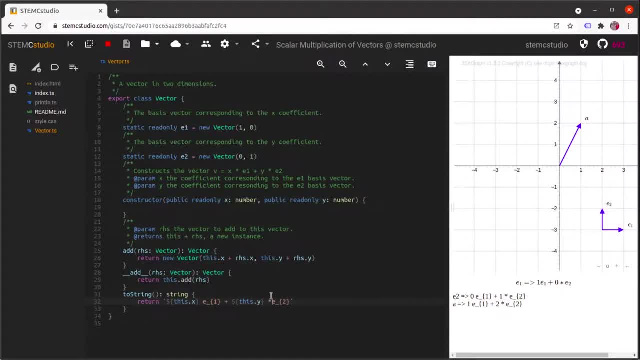 to have this multiplication symbol anymore. So now we got one E1 plus zero E2.. And you can obviously see that. you know that we could really improve this two string, because you know the zero, we don't need to know about it, And one is just one, It doesn't change anything, And so you know. 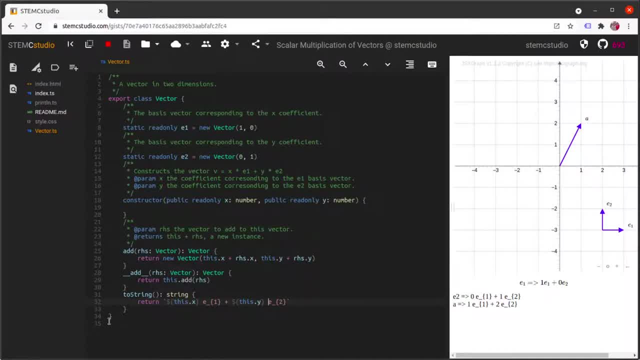 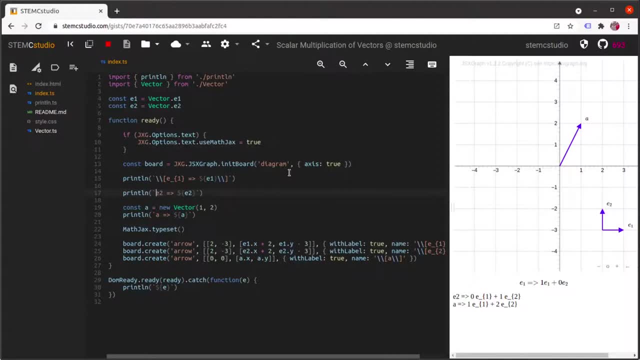 E1 is just E1. No great surprises, But we'll get to that, Okay. So let's go back and just pretty up the rest of it. So backslash, square there, Double backslash, Close the brackets, And there's the E2.. And then, finally, just the A. 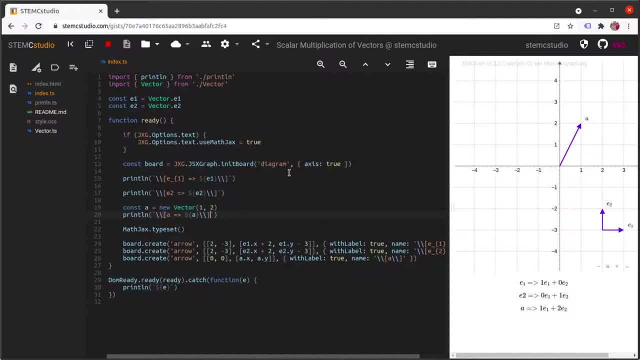 And so A is 1E1 plus 2E2, which is just really what it was defined to be above. Recall that this constructor constructs the vector, which is X times E1 plus Y times E2.. So we expect it to be: 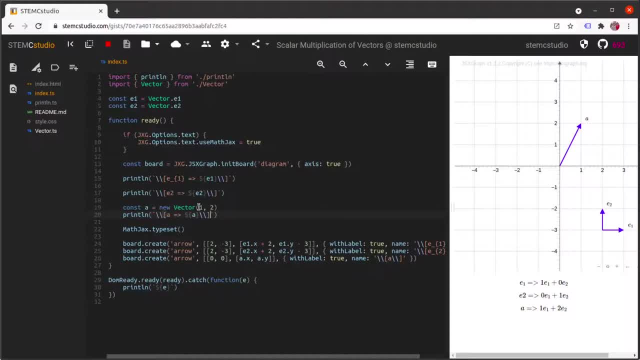 1 times E1 plus 2 times E2, which indeed it is Okay. So two things that we just did there: One is that we used MathJax And one is that we just improved our documentation of the class so that we got better documentation when we're. 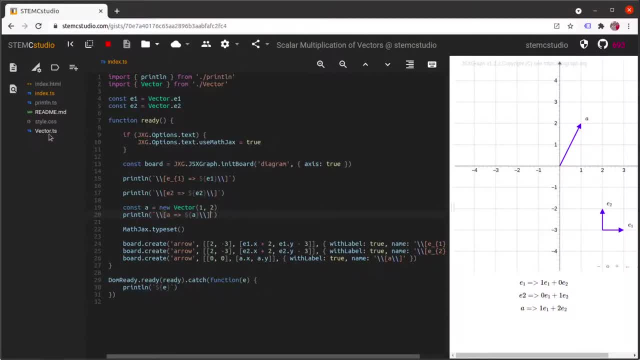 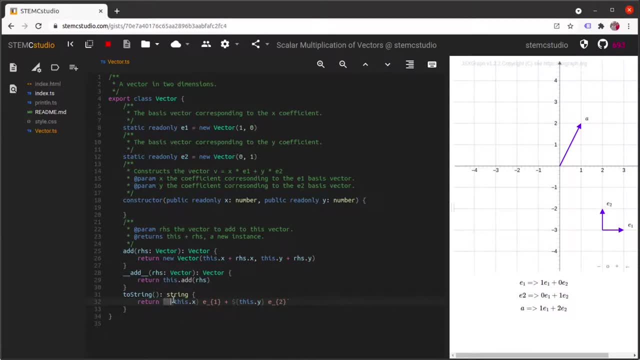 hovering over it. Okay, I now actually just recall. there's one thing in the last video that I was sort of reaching for- I couldn't remember the term. When we have a string like this, okay, and then we embed the syntax with the dollar, curly braces and then variables, we want to 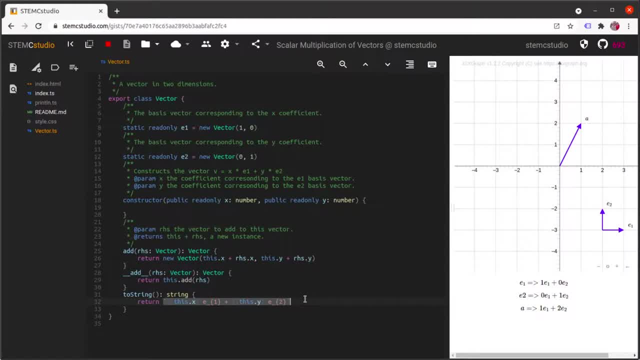 substitute. This is called string interpolation, Okay, Which just basically means that it's going to substitute values into the string And you don't have to kind of like explicitly go and build complicated kind of concatenation statements, Okay. So it's just a very nice, elegant way to work. 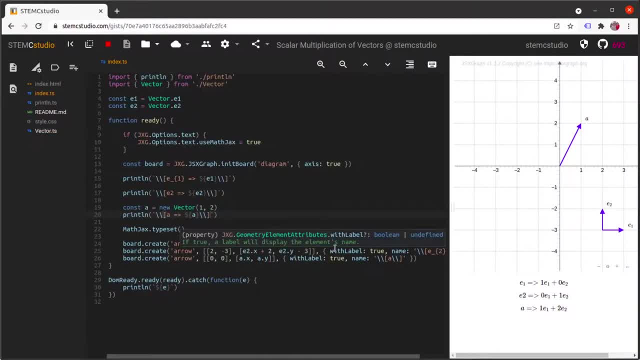 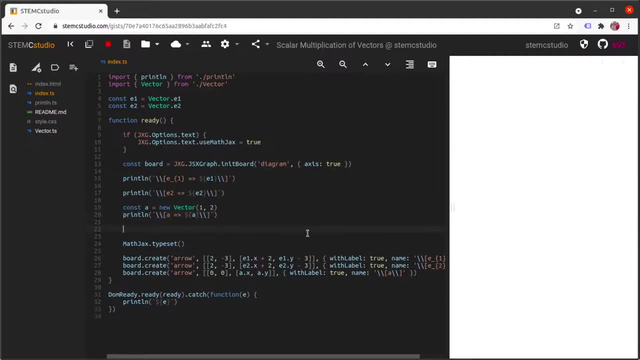 All right, Let's get back to the business of scalar multiplication. What we would like to do is we would like to do something like this: We'd like to create, say, a new vector, And I'll use the word 2a equals, say, 2 times a, Or we might want to do something like a times 2.. 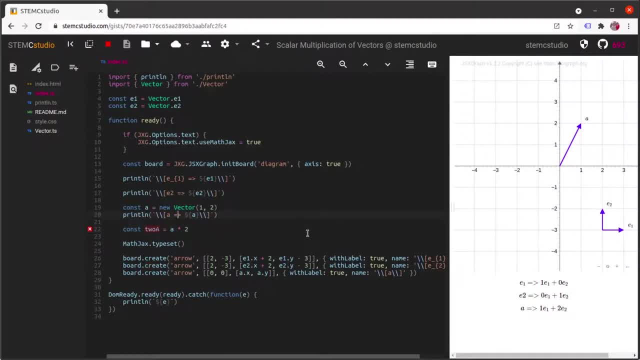 Something like that: Okay, 2a is obviously not being used right now. Let's have it be used So we can say 2a is equal to, and it's equal to, 2a. Okay, So let's say 2a is equal to 2a. 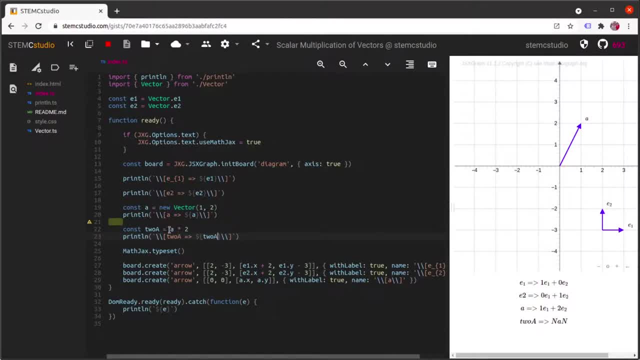 And clearly we're not going to get anything right now because we haven't overloaded the multiplication operator. when it happens with a vector on one side, That's a Okay. Trying to hover over there for you Can't get my mouse in the right place. 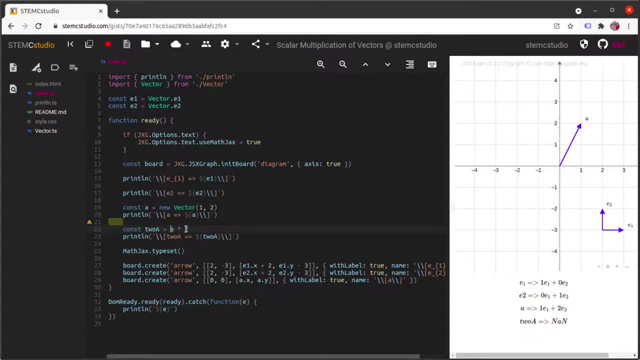 There we go. a is a vector on one side And this on the right hand side. we probably won't get anything, but it's just a number, Okay. So that's not being defined. We also would like to do something like this. 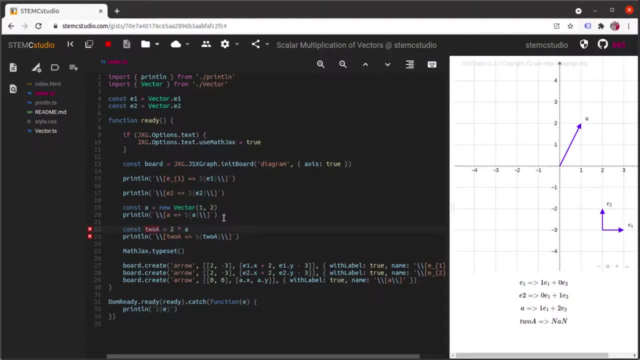 We would like to do something like this Boom to do, as i said, two times a. where the a now is, the vector is on the right hand side and the number is on the left hand side. these are slightly different, so that's what's going to make operator overloading. 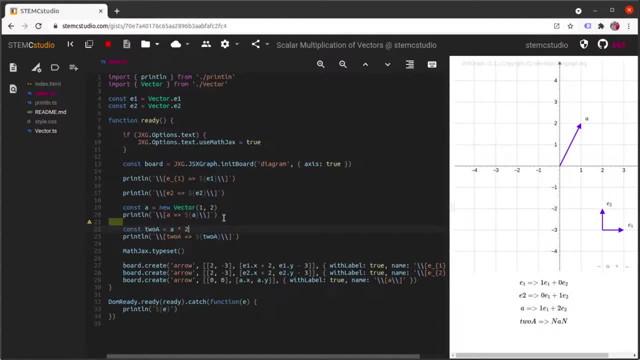 for these today, a little bit different from what we did last time. okay, but like we did last time, let's kind of like do a little prelude and let's do a dot multiplied by: say: well, i'll create a method called multiply by scalar and we'll multiply it by number two. okay, multiply by. 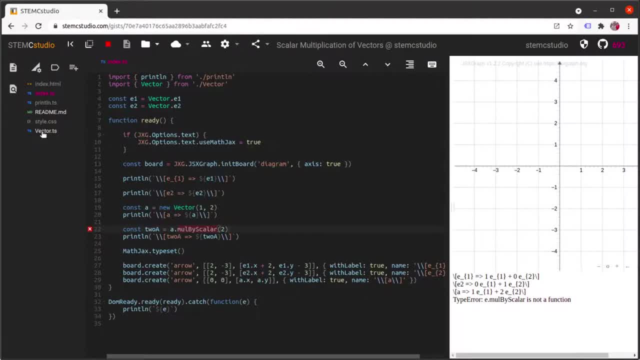 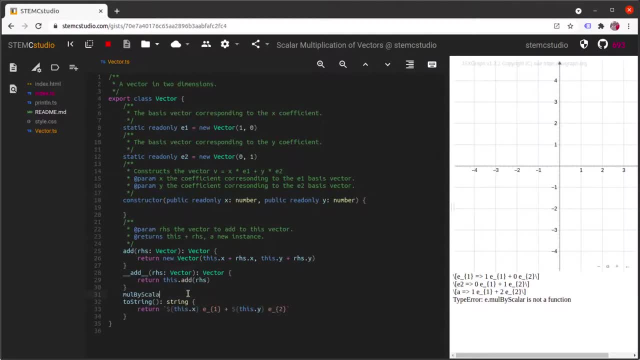 scalar doesn't exist, so let's go and implement it. here we are in our vector class. we can put mol by scalar down here, and the scalar alpha is probably a suggestive number, and this is going to return a vector. oops, okay, so implementation of this should be pretty simple. if you would like to um. 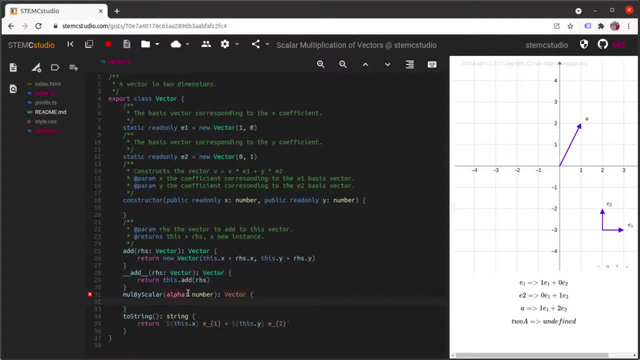 pause the video and try your own solution. now go ahead, but i will carry on. so here, all we really need to say is: okay, this number, by the way, on the right hand side, i think, i think, um, it doesn't matter whether the scalar is on the left hand side of the right hand side. 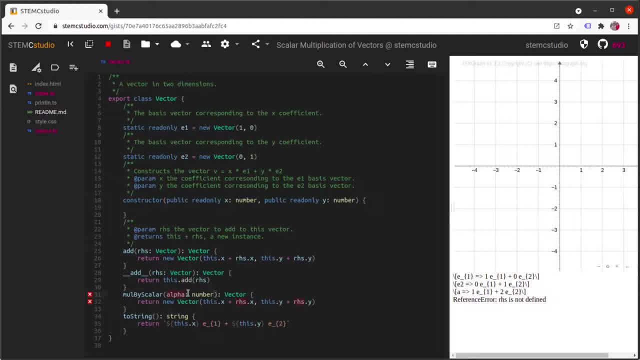 the scalar is on the right hand side, the scalar is on the left hand side, the scalar is on the left hand side of the right hand side. so that's uh and uh. so an axiom of scalar multiplication is that two times a vector is the same as a vector times two. in other words, when a scalar multiplies, 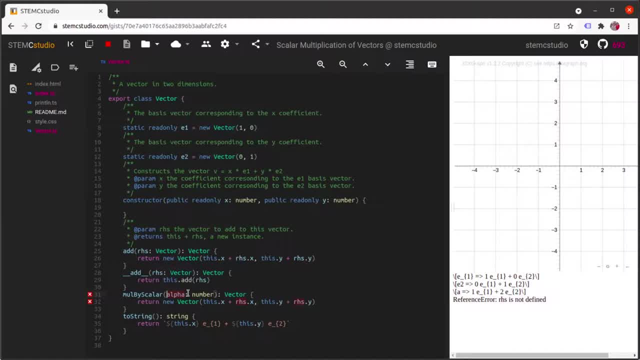 a vector. the result is what we call commutative. that means we can come, commute the two things, we can switch them and it's still okay, okay. so i am going to say: this is this times alpha and this dot y whoops, make sure you get your operator right. 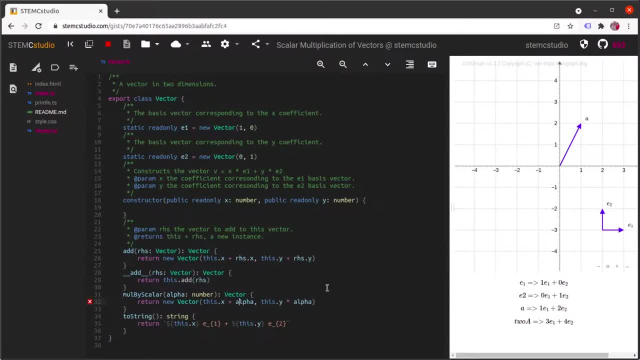 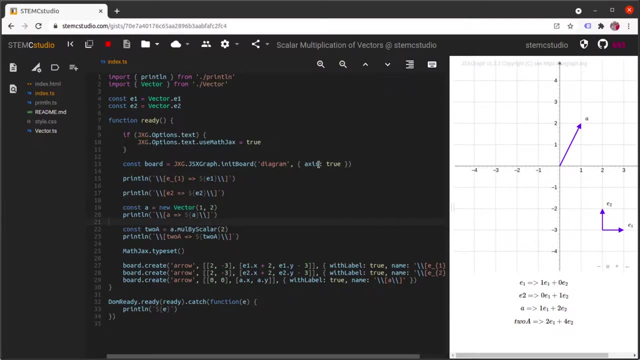 we'll do that again: this dot x multiplied by alpha and this dot y multiplied by alpha. let's go back mole by scalar. so there's the mole by scalar, just get a little bit of white space or format document. so 2a is 2e1 plus 4e2. 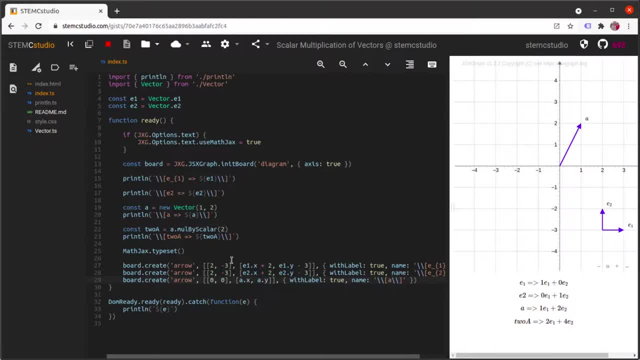 great, that's what we want. let's go and visualize that too. so we'll go board, create arrow, and we want to visualize the vector, which is 2a, and we'll leave it positioned as you can see. we'll start at the origin. 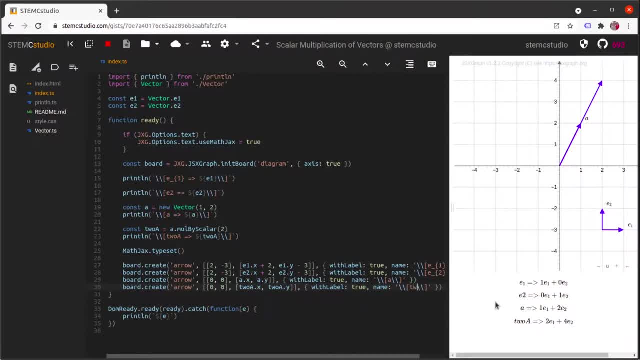 and it's going to be called 2a, whatever that looks. ok and that's kind of what we want. the vector which is 1e1, 2e2 and 2a is 2e1 and 4e2,. great, so we're. 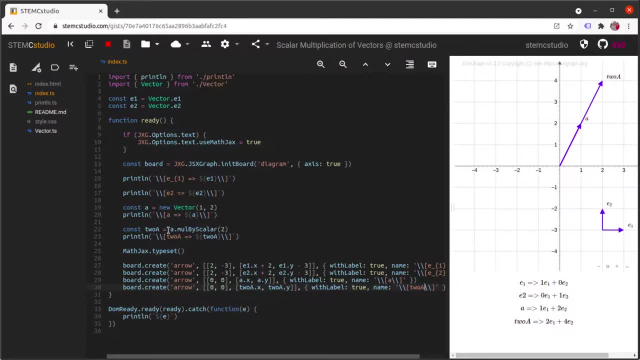 sort of off to a good start, but what we want to do now is we want to replace this multiplied by scalar with something that looks a little bit more like math, so we want to evolve from that to something that's more like a times 2. 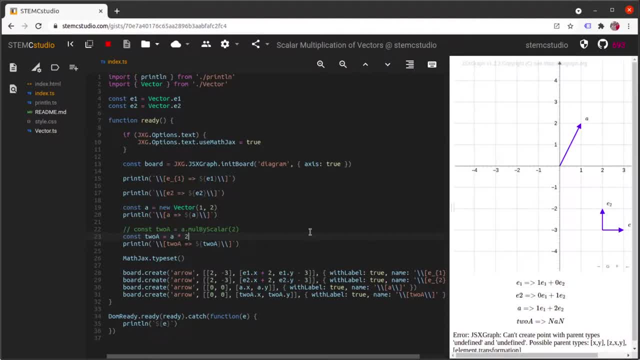 ok. so notice that in this case, before we actually go and implement this, that a is on the left hand side and the 2 is on the right hand side. ok, so the number that we're trying to multiply is on the right hand side. so let's go to our vector class. 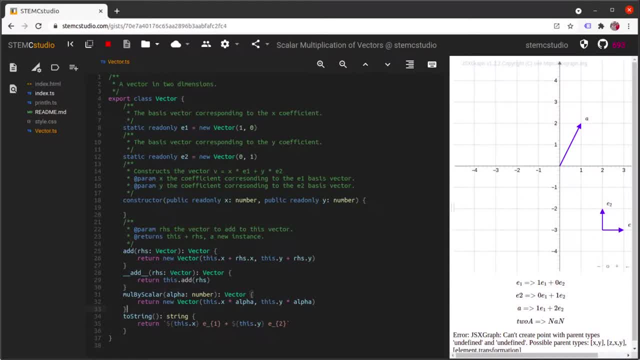 and we want to overload the multiplication operator, so the the, the method that we need to define, is called mul. ok, and the right hand side, as I said, this time is a number and what it's going to return is a vector. ok, and then, just as before, 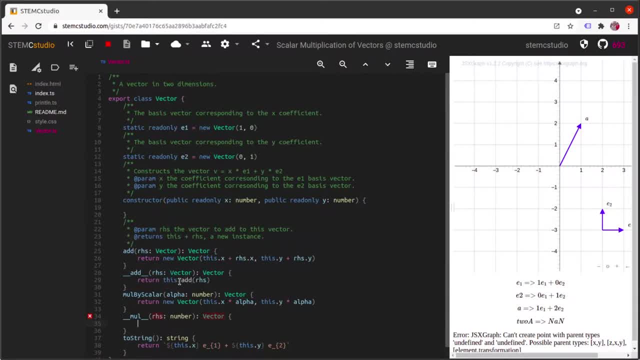 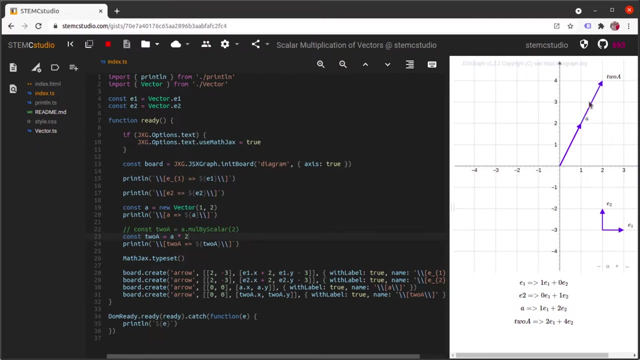 where the add method could reuse the thisadd. we can reuse thismul by scalar and we put the right hand side in. ok, and just do a little formatting. let's go to our main line and, as you can see, it worked. we've got a there. we've got 2a there. ok, let's do the. 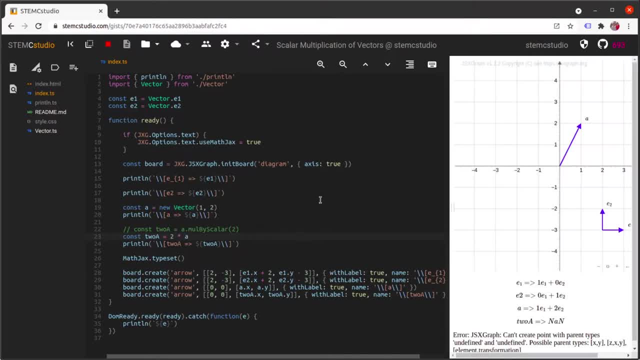 other way. let's do 2 times a ok, and then once again you can see that it didn't work out. nothing's been evaluated ok. that is because we have done a pretty simple multiplication for the right hand side, for the left hand side. 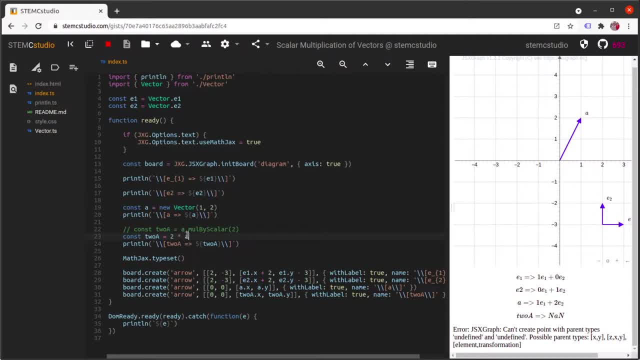 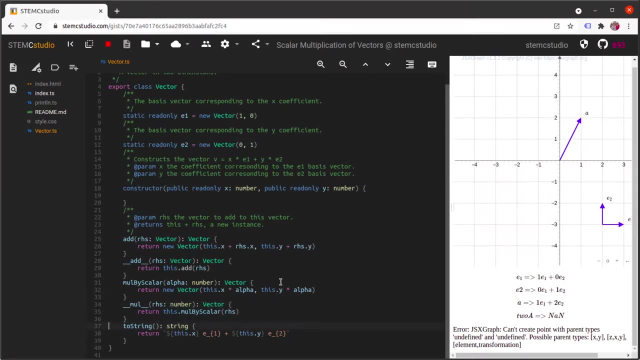 and what we need to do is implement a slightly different operator overload, where now the a happens to be on the right hand side. ok, so that method that we implement is called right multiplication. so we are going to have an Rmul, ok, where 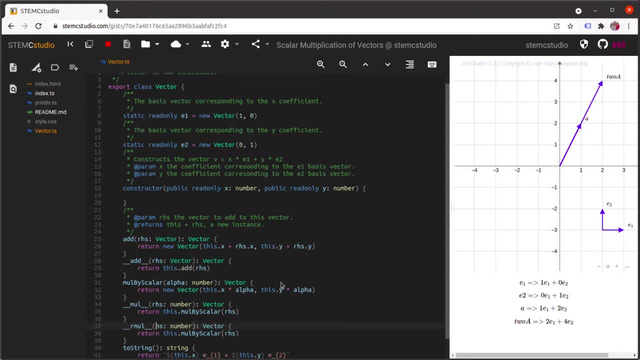 the. the number that we want to multiply right right now is on the left hand side. okay, and we are on the right hand side now. this is not important for scalar multiplication because we know it commutes, but going forward with geometric algebra it's going to become very 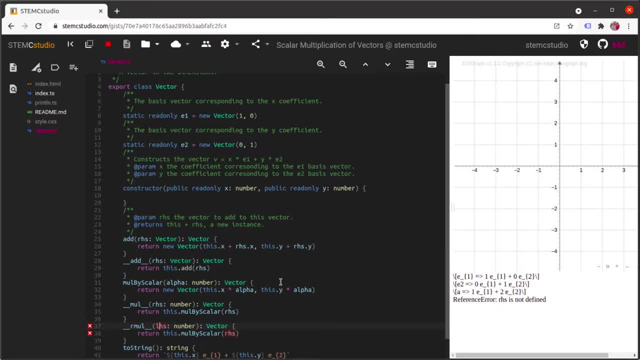 important. so, in addition to making this work, you should start to question: every time that you do multiplication, am i allowed to flip the um? flip the two operands in my expression. an example where you can is like addition um, an example where if you flipped it um, it would give. 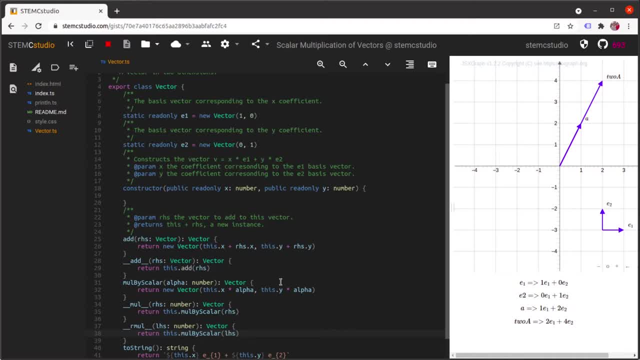 the wrong sign would be subtraction. okay, change the ordering. a minus b is the negative of b minus a. um, there are going to be other operators, though. when we we come, come across them where, if you reverse the or the, if you change, interchange the two operands, the two things that 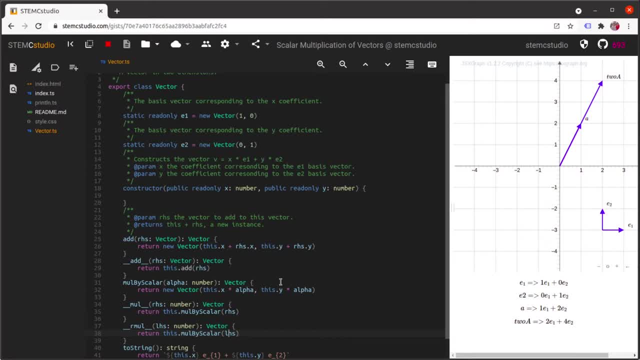 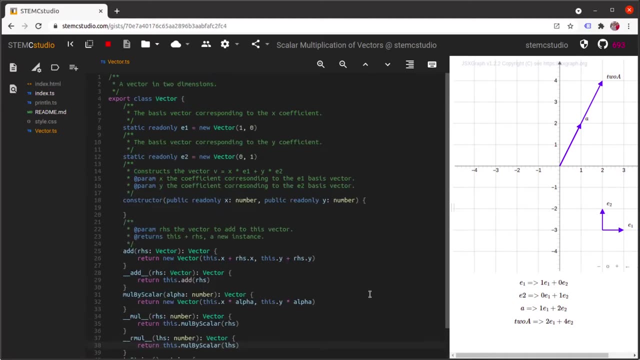 are being operated on, you'll get some kind of completely different answer. okay, so just look for that as we go forward in future. so the good news is that we actually now have scalar multiplication, um by a vector. we have implemented um also mathjacks, so we've got sort of rather 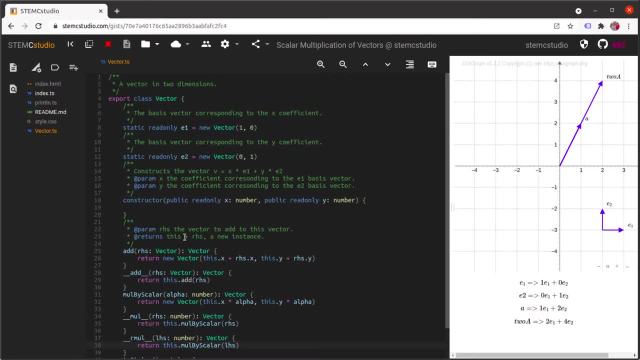 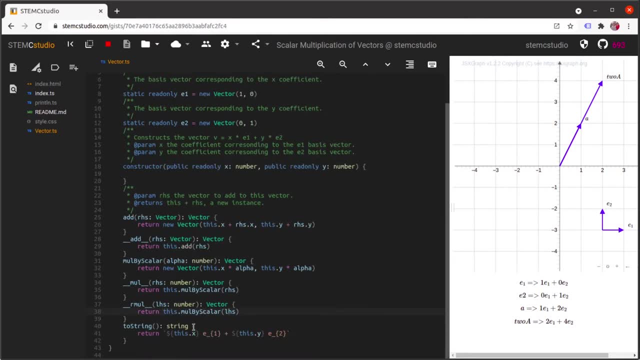 more elegant output here, and we've also learned a little bit about using the javascript documentation to improve our code. i'll leave it as an exercise for you to document the mul by scalar method and the two string method, um, to just make those a little bit more friendly for. 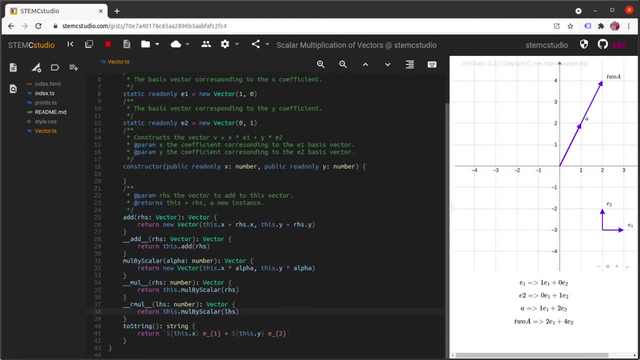 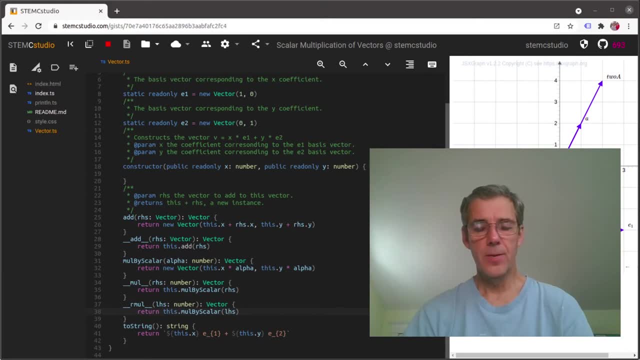 for anybody who wants to use them. i hope you enjoyed that. uh, very um video, a relatively short video. um, this video has moved us. um, moved us along a fair way with our vector, but there is still more to do with with vectors. um, we have yet to define anything related. 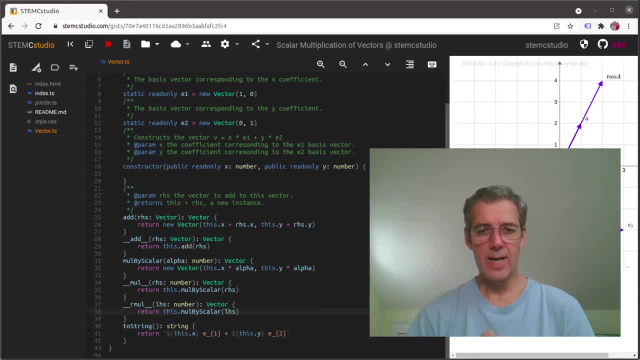 to the magnitude of the vector. um, we don't know how to compute angles between vectors. and then there are many, uh, there are a few other little odds and ends that we want to, uh, just tidy up before we're done with the vector. but we will be able to move on very shortly to turning this into what i would call a geometric